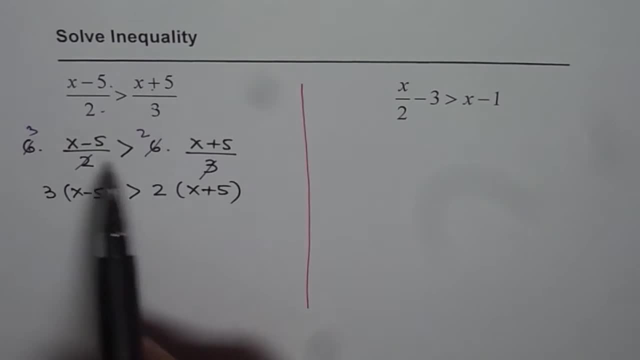 one thing: Both are positive. If one of them, or if the product is negative, then you reverse the sign also. Now let's expand and simplify. So we get: 3x minus 15 is greater than 2x plus 10.. 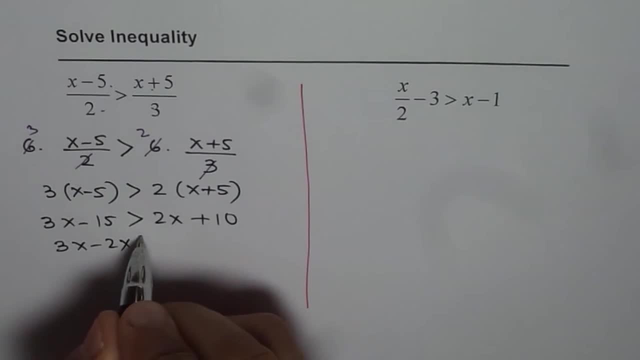 Multiplying the terms together, 3x minus 2x, is greater than 10 plus 15.. So it is x greater than 25.. Now you can write answer x greater than 25.. Sometimes you may have to represent the answer on a number line. In that case you can draw a number line and: 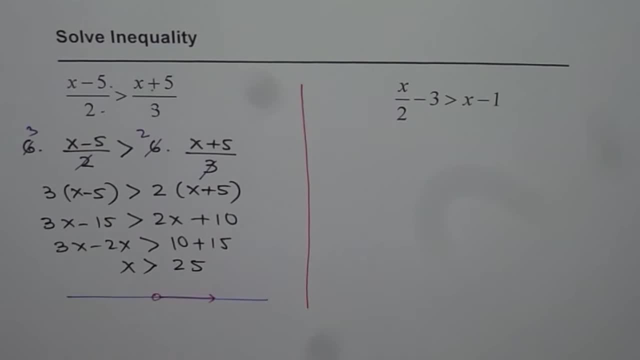 say: well, this is not included, which is the point 25.. And the right side of 25 falls, the solution set. So that is the point 25.. Here, let us say we have a 0,, which is not a part of solution. You can always test If. 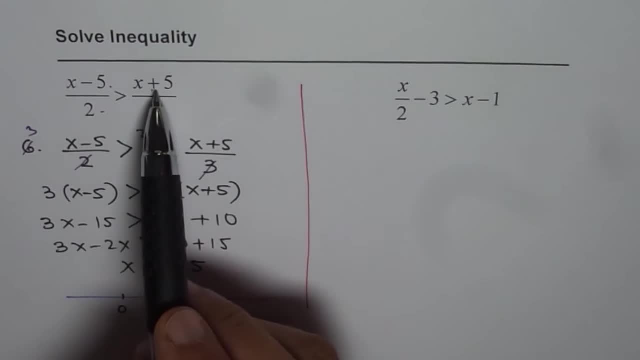 I plug in 0 here. I get minus number here, positive number here, which is definitely not greater. So that is not a part of solution set. So that is how you can check. Now you can pause the video, copy the question and solve it on your own. The strategy is: 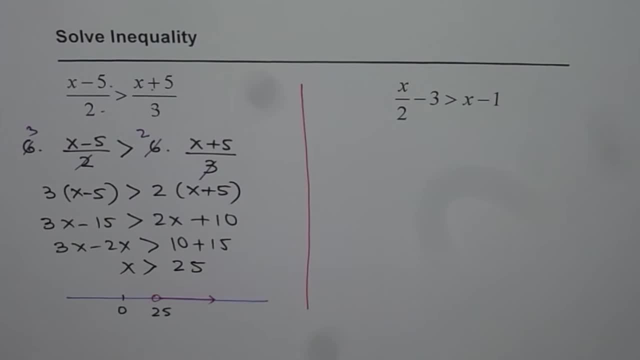 what we did. Now. here is my solution. Now again, we will follow the same method: x over 2.. So what we have here is a fraction again, So you can multiply everything by 2, but this is very simple, So doing that may not be advisable. So what we will do in this case? 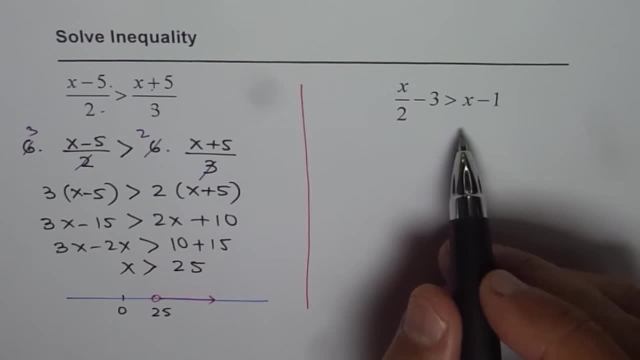 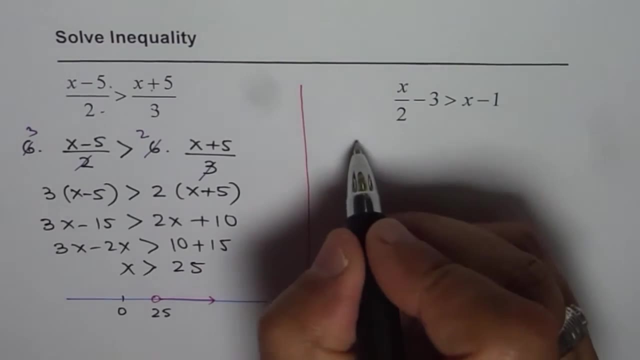 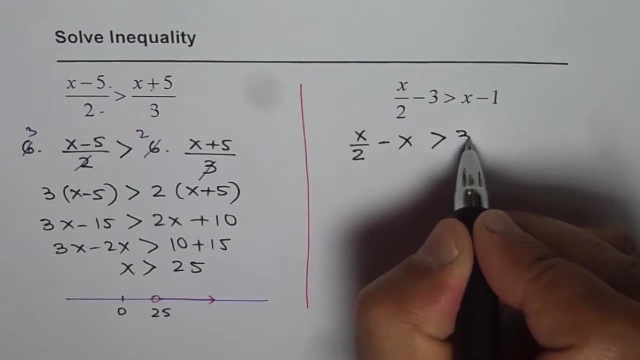 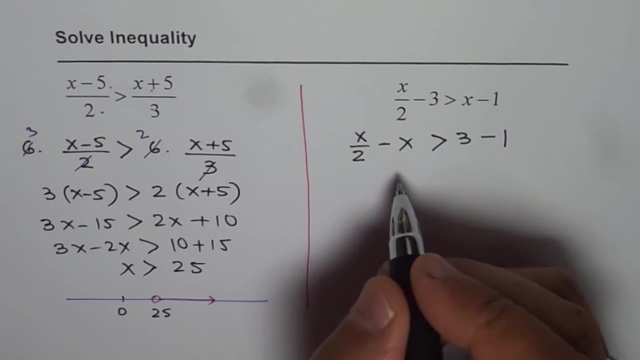 is, we will take the numbers together and the variables on the left side and then solve. So we can write this as x over 2, take away x greater than if I take 3 on the right side, it becomes plus 3, minus 1.. Now x over 2 minus x is minus half x, Or you can take common. 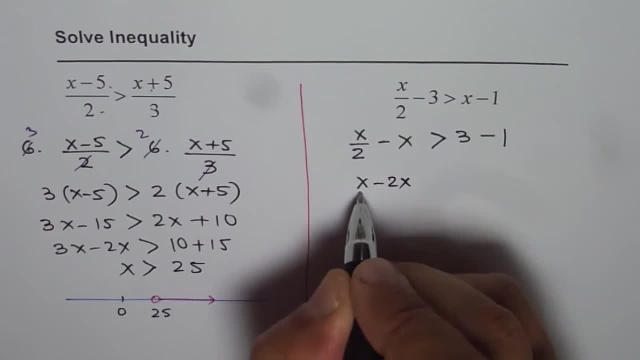 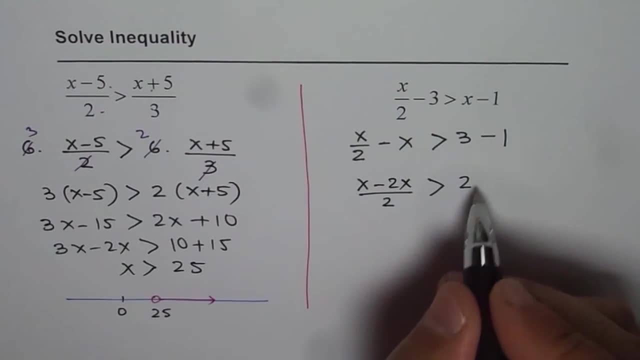 denominator and do it This: x minus 2x over 2 is greater than 3 minus 1 is 2.. Now you can multiply both sides by 2.. So what do we get? Or what we can do is, we can simplify. 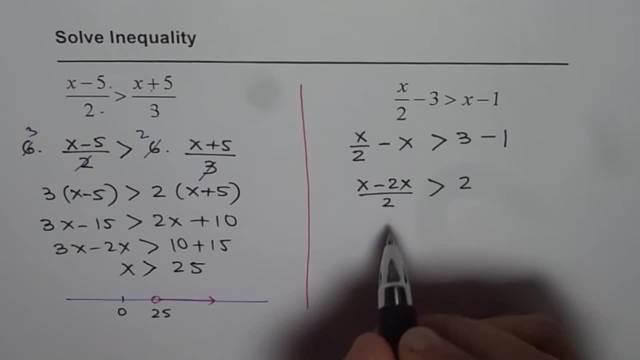 the numerator x minus 2x is 2.. So we can write this as x over 2 minus x. So let me write this as minus x by 2 greater than 2.. Now to get x, we should multiply by minus 2.. So what we should do is multiply. 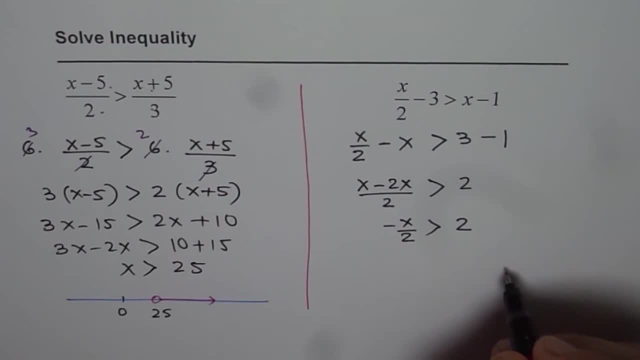 by negative 2.. So when we multiply by negative 2 on both sides, what should we do? So you are doing times by minus 2 both sides, right, Remember one thing: whenever you multiply by a negative number, you have to reverse the sign. So this was kind of very critical. 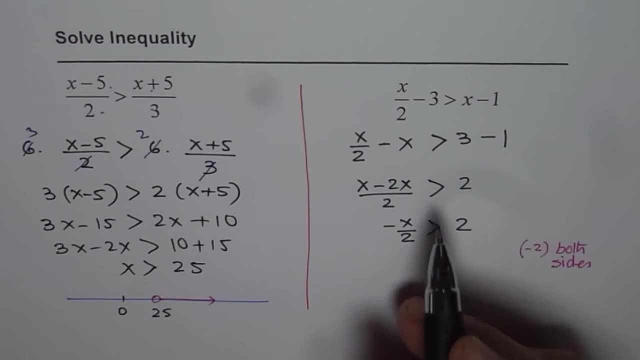 for me to explain you, and that is why I was taking time to solve it. Now, if I multiply by minus 2, I really get minus 2 times minus x over 2 and I have to reverse the sign. Let me reverse it: 2 times minus 2.. Do you see that Now, minus 2 times minus x will become. 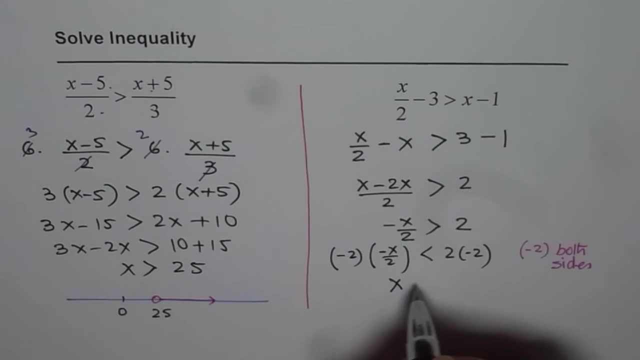 plus 2x, and 2 divided by 2 is 1.. So we get x is less than minus 4 as your solution. Do you get it? So that is how we find the solution. On a number line, you can represent this solution. 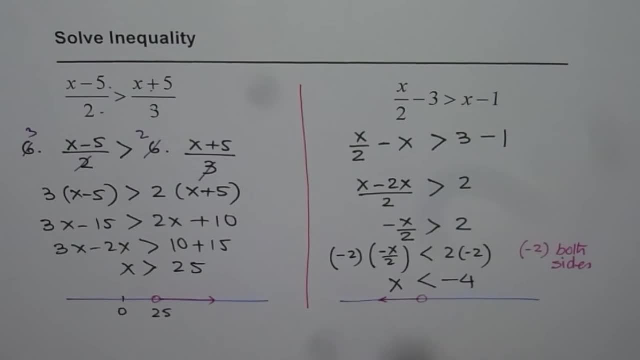 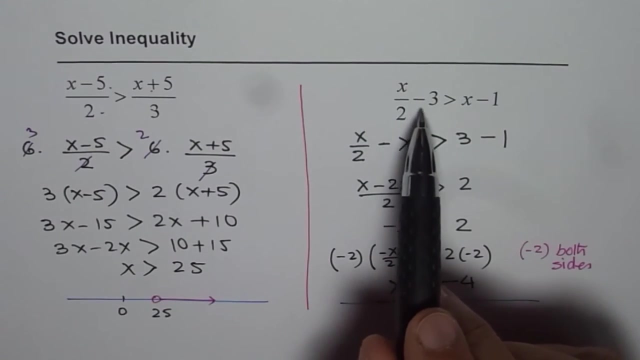 as x is less than minus 4.. Let's say this is 0,, which is not a part of solution. So if I write 0 here, this inequality should not be satisfied. So what do I get? I get minus 3,, which is minus 3.. Minus 3 greater than minus 1,, which is incorrect. But if 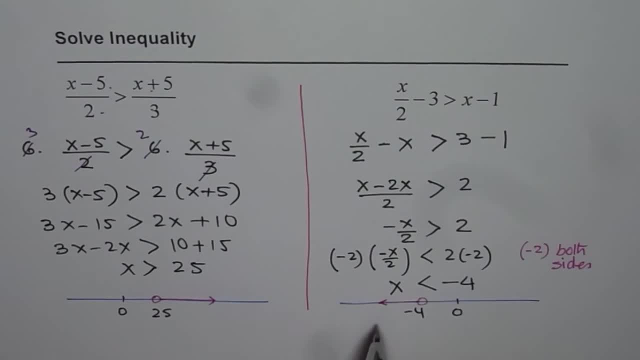 I write a number which is on the left side, a part of solution, which is minus 6, let us say, Minus 6 divided by 2 is minus 3.. Minus 3 minus 3 is minus 6.. Now, if I do greater, 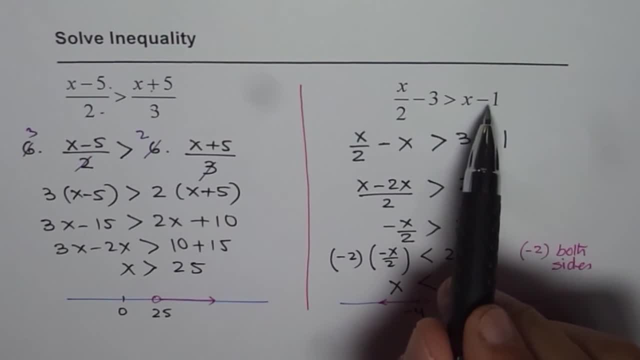 than minus 6, minus 1 is minus 7.. So minus 6 is indeed greater than minus 7.. That makes the inequality true. So that is the correct answer. So the solution is right there for you. That is a part of.